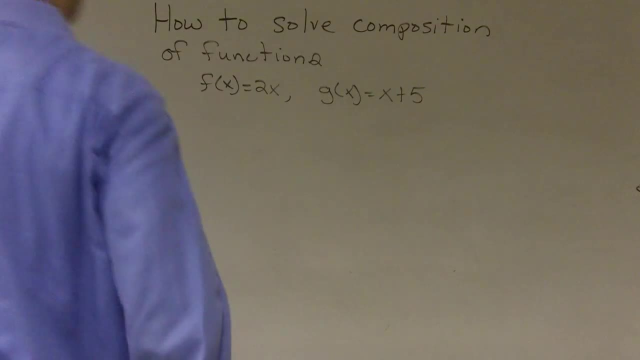 What I like to do is show you guys how to solve a composition of functions. So essentially what we're going to do is we're going to find f of g of x and g of f of x, And the thing that gets most students is kind of like the notation. So, if we can kind of take a step back, we're going to do a quick review. If I was given f of x equals 2x and then I said, well, 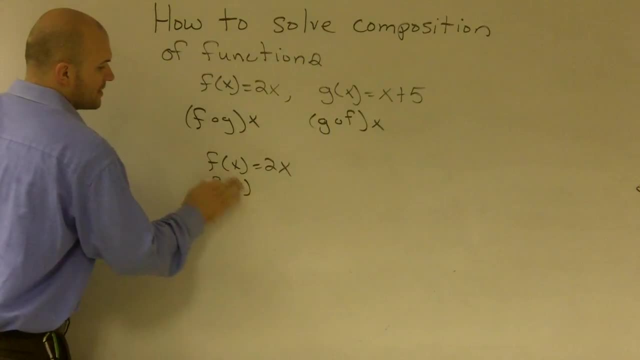 if I want to find f of 2, let's do f of negative 3.. We remember that your x, this is a function. you have an input and output value. So whatever you plug in for your fx, that's what you're going to plug into your function. So my negative 3, I'm going to put that into my function. for my x, So it's going to be 2 of negative 3.. So we can evaluate: f of negative 3 equals a negative 6.. And then now that is my output. Remember function. you have your input, your output. 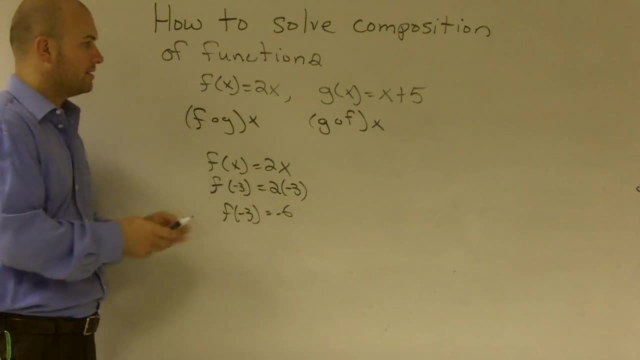 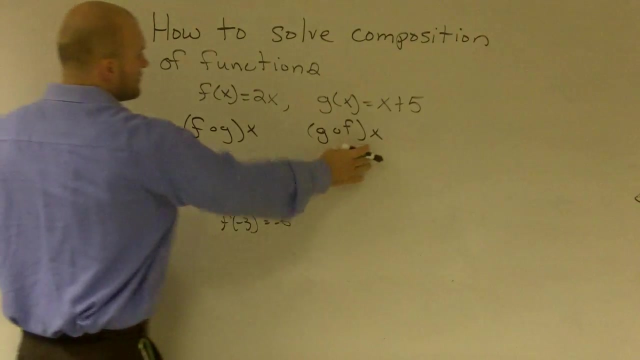 Whatever is in here, that's what you input into your function and then you'll get your output. Essentially, we're doing the exact same thing with here, except now we're using two different functions. So let me go and do this one first. So when we have the g of f of x, it gets a lot of students confused because they don't really know what that relates to. So let me rewrite it in maybe different terms. Essentially, g of f of x is g of 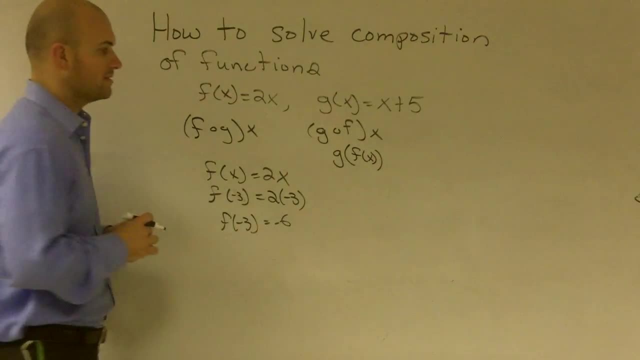 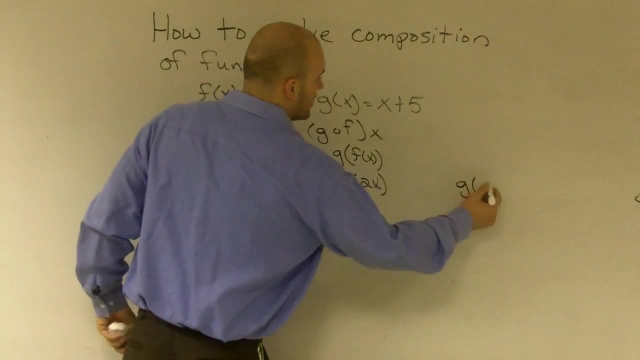 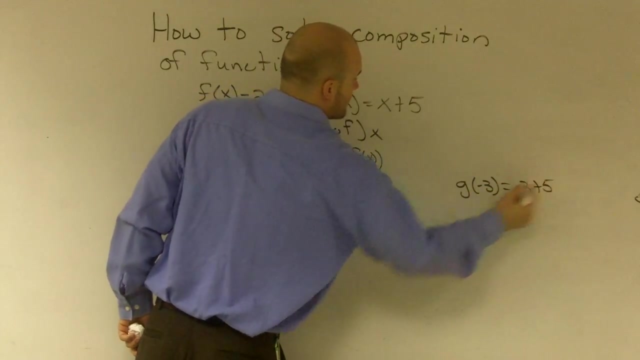 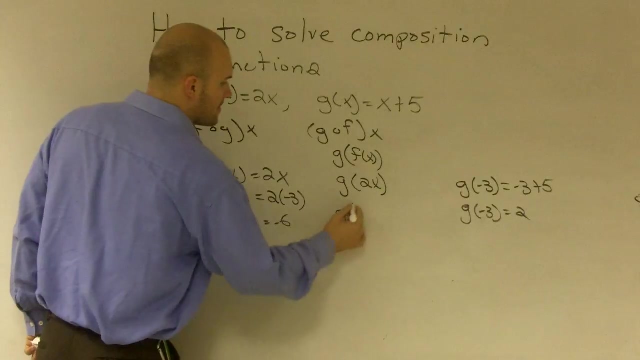 of negative 3. The g of g of negative 3 is g of negative 3. So g of g 3 plus 5. so g of negative 3 equals 2 over here. g of 2 of X equals 2x plus 5.